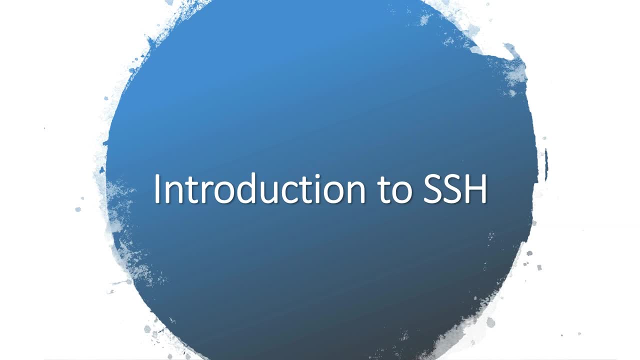 RSH for remote login. So you might even run into an issue where you're using a program such as Telnet, where it's very easy to crack the username and password without being detected. How can these serious problems be prevented? One of the ways you can prevent these is by 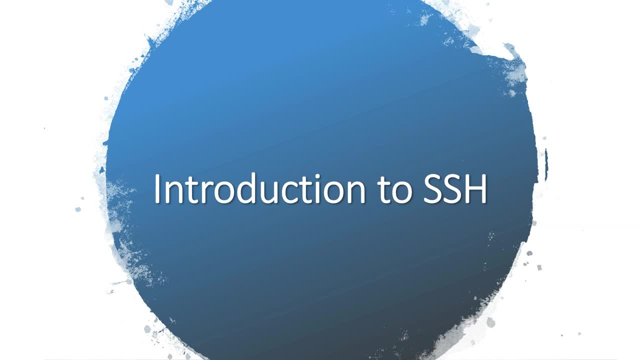 using what is known as the secure shell. You can use this encryption program to scramble your data into a secret code that nobody else can read. Sometimes you can install a firewall on the device that shills portions of the computer network from intruders, and 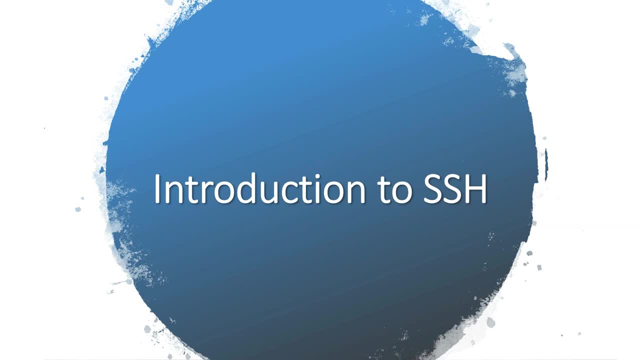 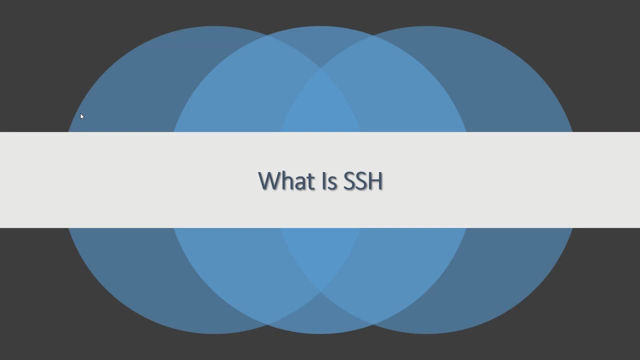 keeps all of your communications behind it. But SSH is really the way to go. What is SSH? As stated, SSH stands for the secure shell. It's a popular, powerful, software-based approach to network security Whenever data is sent by a computer to the network. 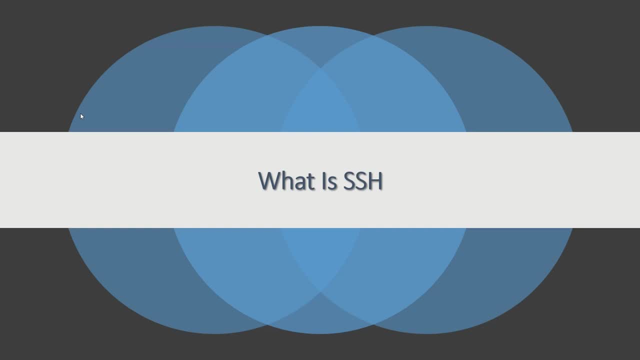 SSH automatically encrypts or scrambles that information. If other users were to intercept it, that data is very well encrypted where the user wouldn't really be able to decrypt it and it would take so long that most hackers would just leave it alone. 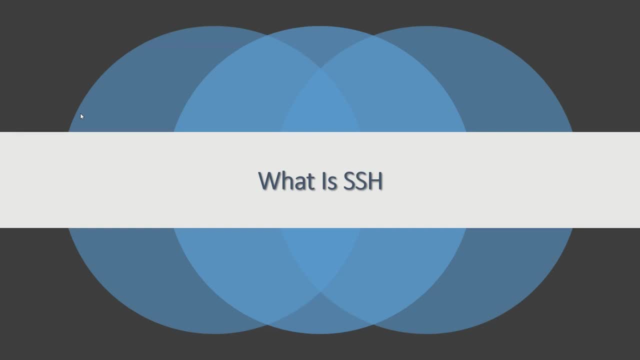 Once the data is scrambled or encrypted. when the data reaches its intended recipient or its intended user, the secure shell or SSH will automatically decrypt or unscramble that data. The result for this is what is known as transparent encryption: Users can work normally without really being detected. 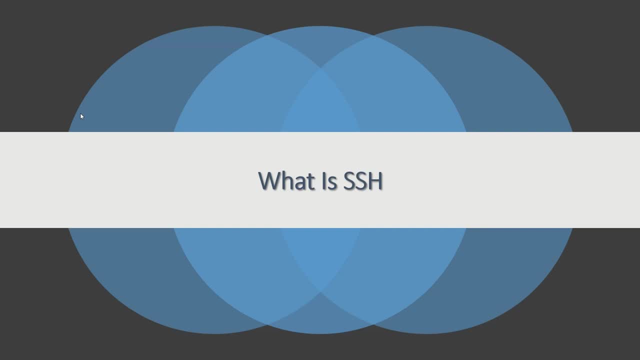 and their communications are safely encrypted via the network. Let's say I'm working in Atlanta. I want to access a computer that's in Boston. I can actually do that without fear of something happening to that machine. The secure encryption that SSH use is very effective. 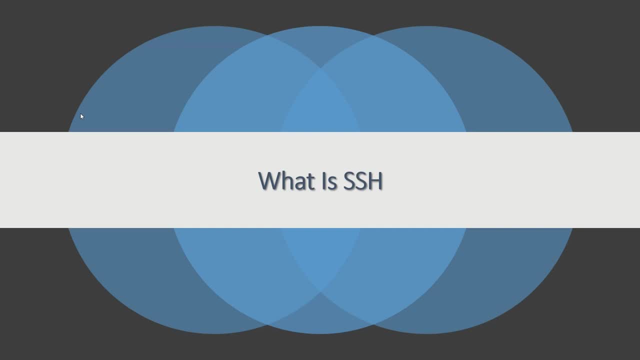 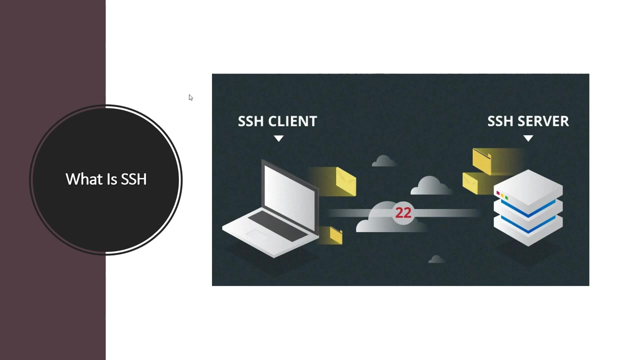 and it's effective enough to be found within, you know, mission critical applications is what I would call them, and many major corporations actually use SSH. okay, So what is SSH? So SSH has a client slash server, as depicted in this image that you see here. okay, 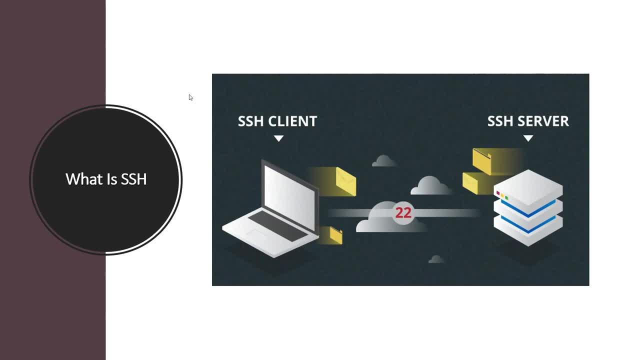 So an SSH server program typically installs and run is typically installed and run by a system administrator. It accepts or rejects incoming connections to its host computer. users can then run SSH client programs, typically on the other computer that's trying to access that particular computer to make the request of the SSH server. 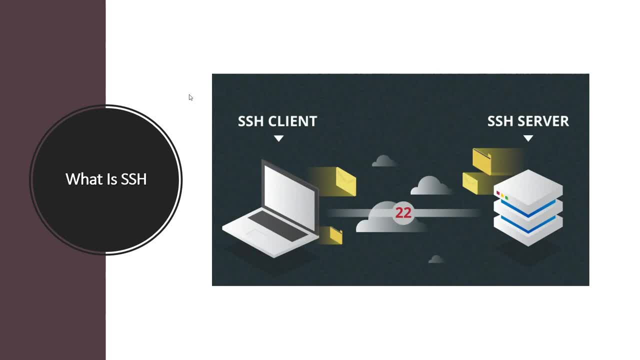 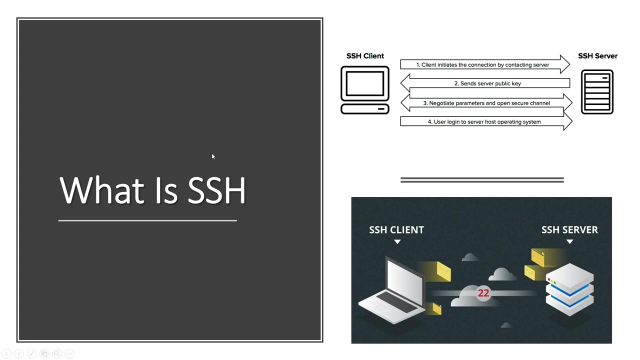 So you can actually make any of your workstations act as an SSH server. Then you would request a login and execute the SSH command to allow for you to securely access and encrypt your connection. okay, So what is SSH? Again, let's take a look at what we're talking about, okay, 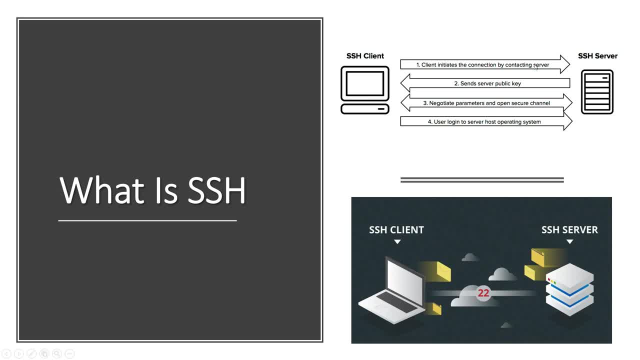 So what is SSH again? So first the client initiates the connection by contacting the server. okay, Think about this as two operating systems, one of them, so two computers, One of them's in Atlanta, one of them's in Boston, or Boston to LA, etc. 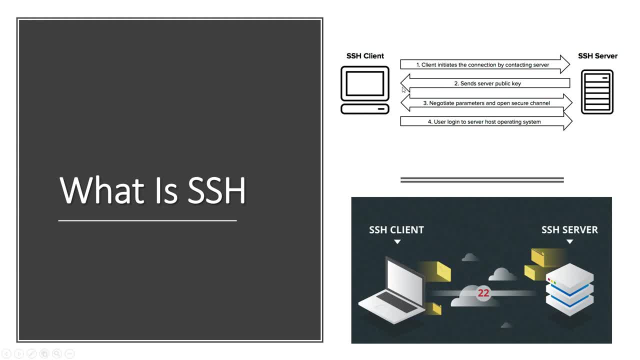 The computer then sends that user server a public key. From there they negotiate the perimeters of an open, secure channel right, But the key is really what's gonna allow us to access that. The user is then allowed to login to the server of that host operating system. 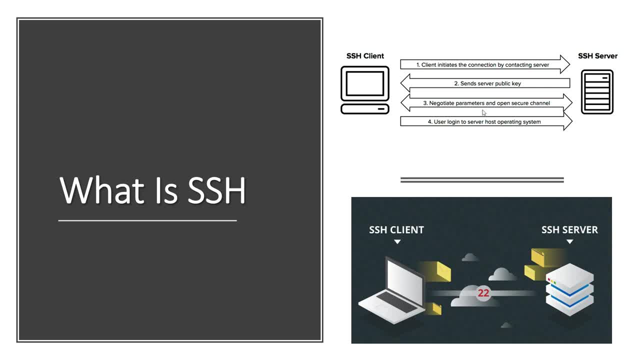 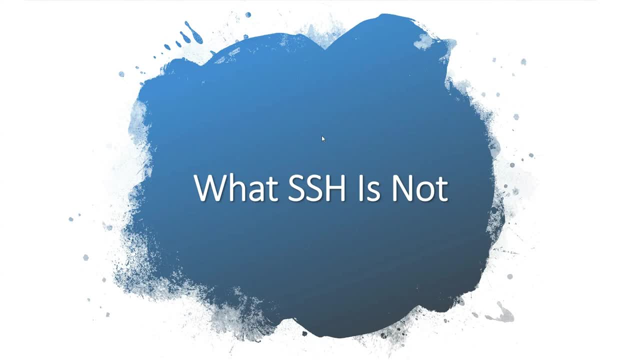 So you can actually access that machine and do whatever it is that you would like to do. So what SSH is not okay. Although SSH stands for secure shell, that is not a true shell in the sense of what many would call the C shell or the Unix type of shell. okay, 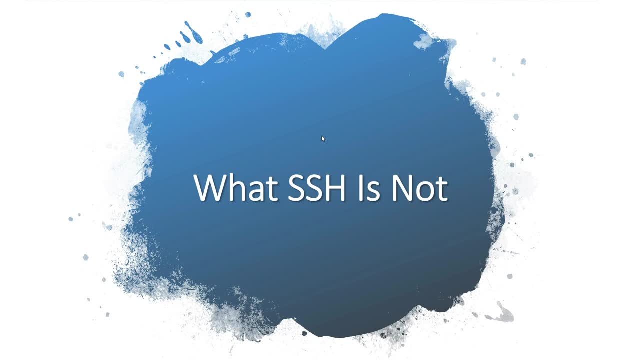 It's really not a command interpreter, nor does it provide what's known as wildcard expansions or command history and so forth. Rather, SSH creates what's known as a channel for running a shell on a remote computer with end-to-end encryption, so point-to-point encryption between the two systems. okay.